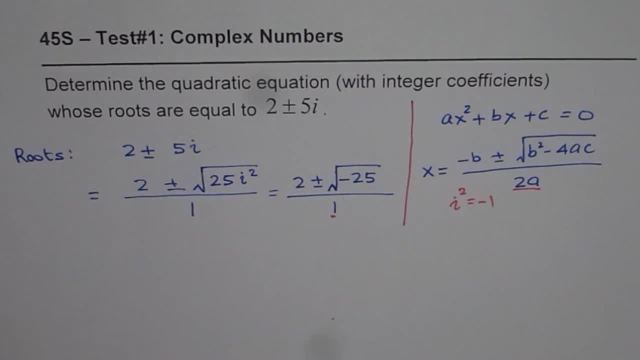 Let's compare the denominators. So if you compare the denominators, we get 2A equals to 1, and therefore A equals to 1 over 2.. So in this equation we get the value of A as 1 over 2.. 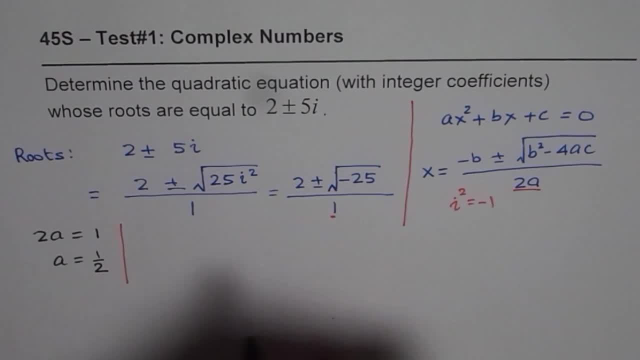 So that is one of the values which we got. Now let us compare this part: B Minus B is equals to 2.. So we get minus B equals to 2, or B equals to minus 2. So we got B also. 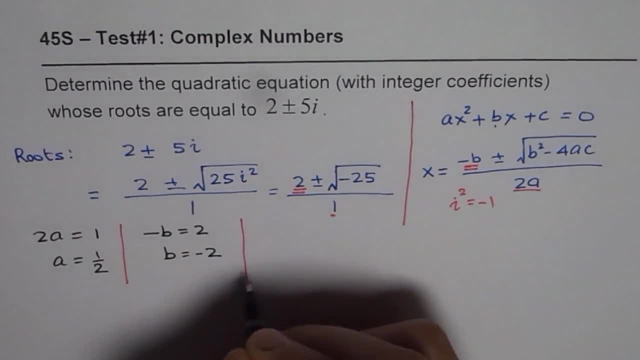 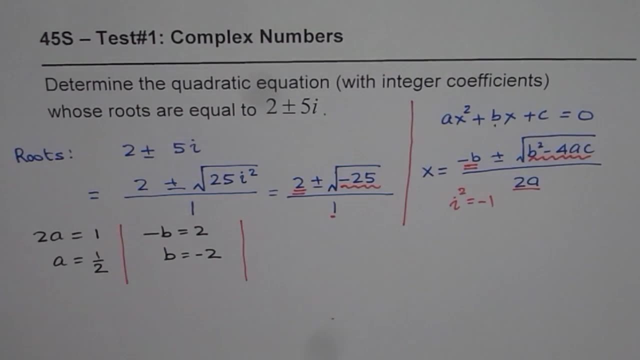 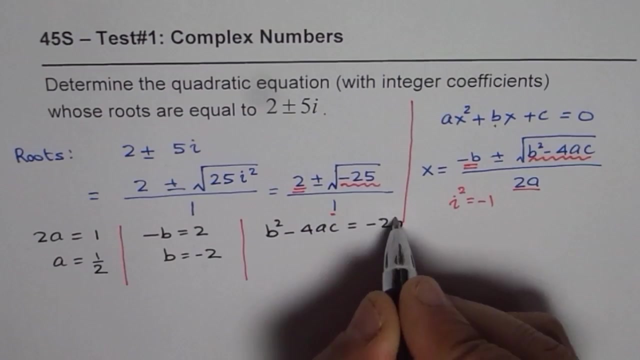 Perfect. So we got two things done, And now let's look into this part. Which is this part? Is that okay? So it says B squared minus 4AC should be equals to minus 25.. That is what it says. Now, what is B? 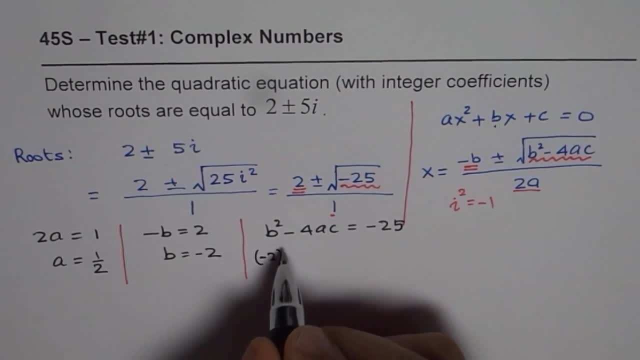 B is minus 2.. So we'll substitute minus 2 here. square minus 4 times A is half Times C is minus 25.. Do you see that Now in this equation we have only one variable which we can find? 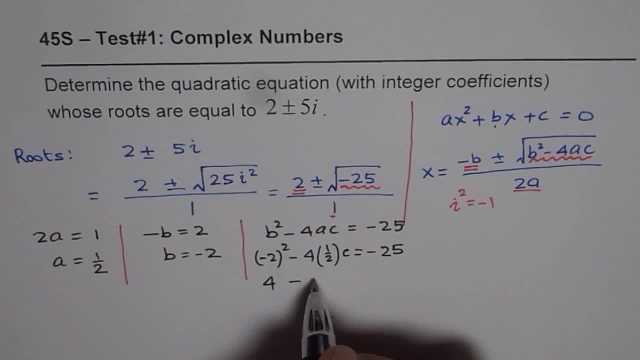 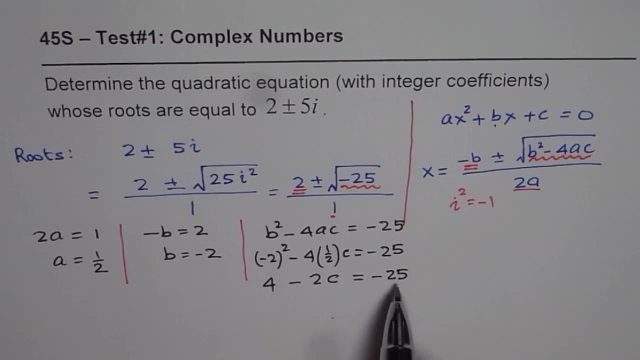 So let's solve for that: 4 minus 4 divided by 2 is 2.. So we get 2C equals to minus 25.. Correct, Now we can rearrange these terms. So we get minus 2C equals to minus 25.. 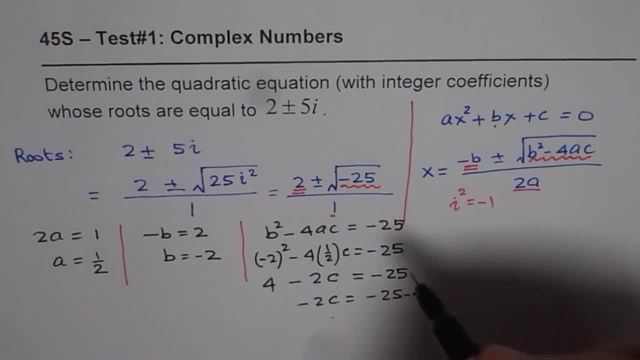 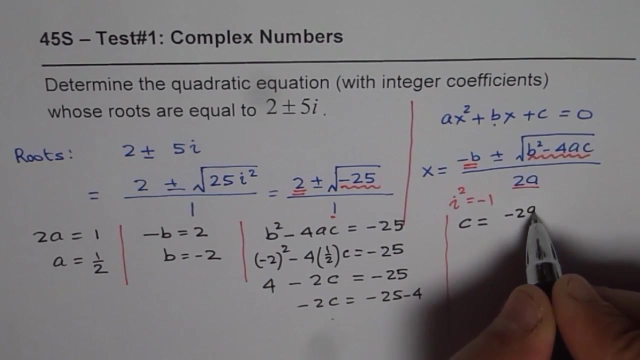 So we get minus 2C equals to minus 25 minus 4.. Let me move to the right further, because I want to just simplify and write the answer here itself, So we can write this as C, as equals to minus 25. minus 4 is minus 29,. divided by minus 2,, minus 2.. 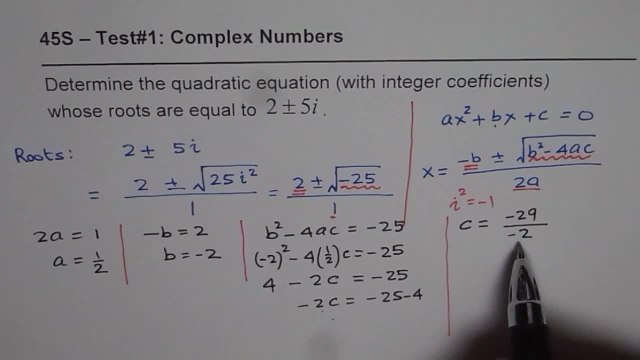 So that is the value of C. Now, once you get the value of C, you know what A, B and C are Correct. Highlight all the things which we found right. So let me write this as 29 over 2..